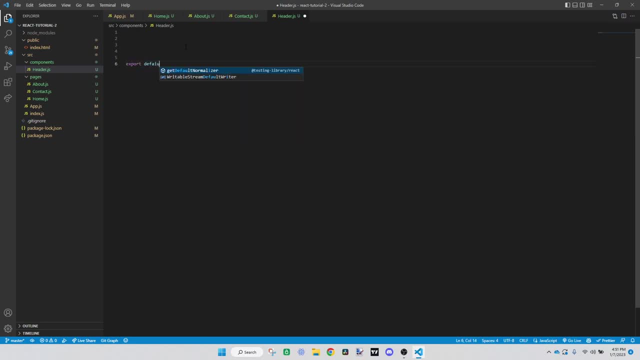 Now in the headerjs we're just going to make very simple, not even really a header, but you get the point. So we're going to create a function header And then we're just going to return a h1 header. react router tutorial. 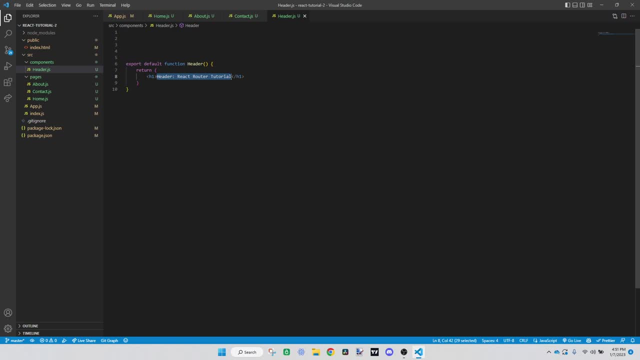 All right, So that's all the header is. It just says header- react tutorial. Obviously, you could have a lot more advanced HTML in here that actually is styled and looks like a header, But we're not going to do that because this isn't a CSS course, this is a react course. now let's go to the pages we're gonna want. 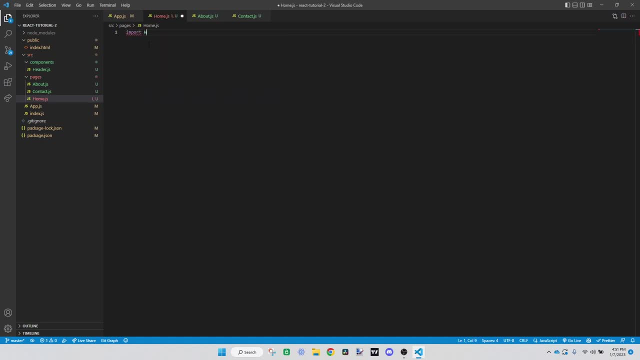 to import that header to put it into the pages. so import header from dot slash components header. it's actually not dot slash, it's dot dot slash because it's out of the same, it's out of the folder. it's one directory back. that's what the dot dots mean. a single dot means it's in the same. 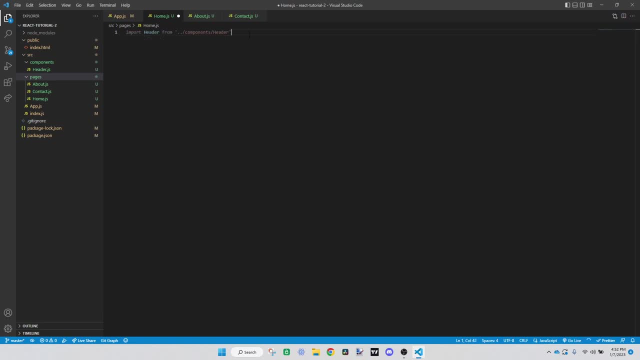 folder. so if you didn't know that, now you know, now we'll copy that, we'll paste it to all the pages and we will go down here and make a component. we'll just return and then we're going to wrap it up and then we're going to put it in the folder and then we're going to. 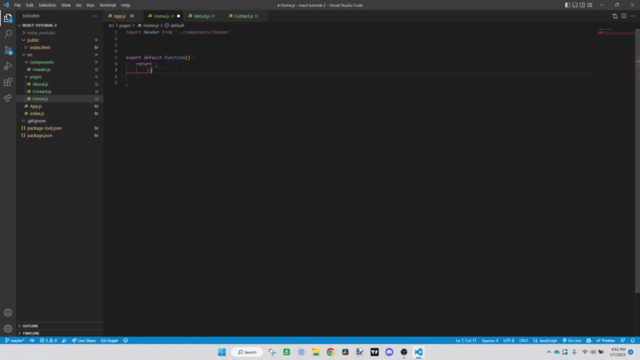 wrap this in a fractal. you could do a div or anything else as well. I'm just going to do a fractal, just cuz. now we're gonna put the header here and then we're going to put h2 home page. now we can just copy this and we can go down here. 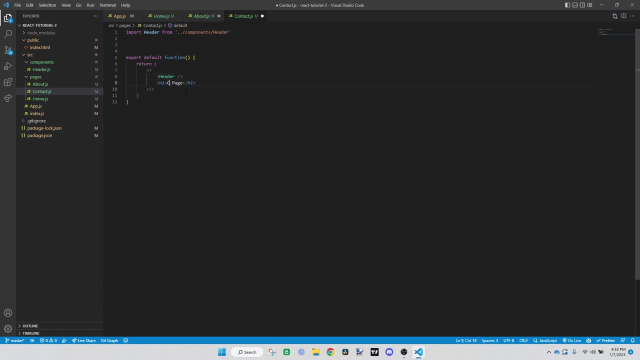 and change the names here. so this is contact will leave header. oh, I didn't even put, I didn't even put a name here. function: contact. there we go. okay, so now we can go over here and change this one about contact and home. so that's all we. 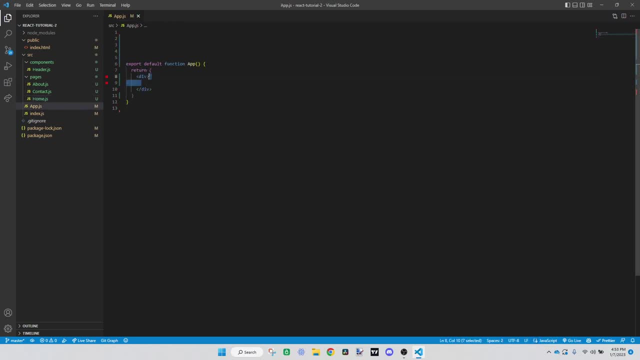 need to do for the pages. you could do again. you can do a lot more advanced stuff there and make it actually look good. but we don't need to make it look good for this video. I'm just showing you how to get it done and you can worry. 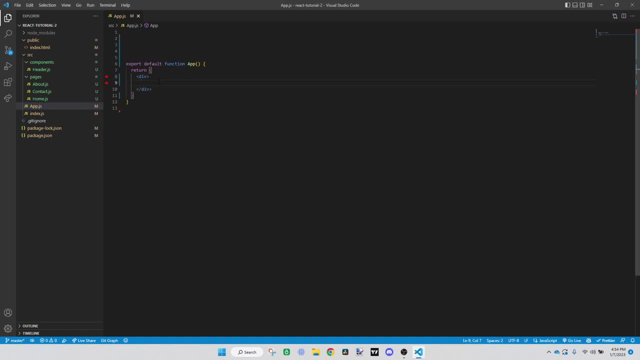 about the HTML and CSS yourself, because that's really all that you don't learn from this, from me not styling it. so now we're going to open the development server. so to do that, you just open a new terminal and type npm- start- make sure you're in the right. 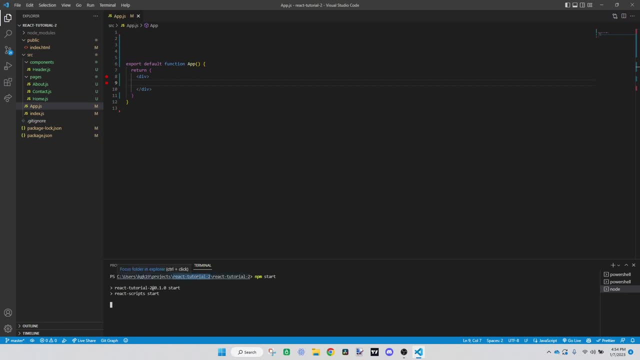 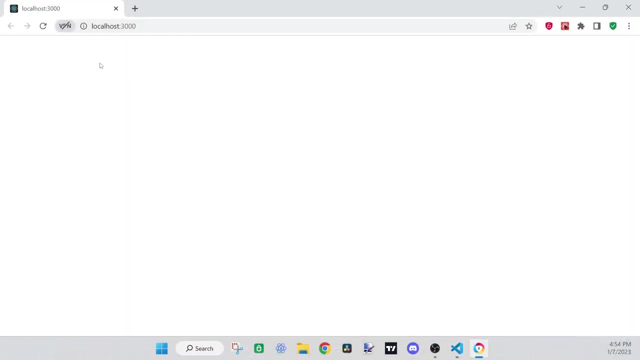 directory. sometimes it'll give you an error. it's usually because you're in this first folder or something and you're not actually on the react folder that it created. all right, so now you can see over here it's loading up and now it's blank because there's nothing shown. 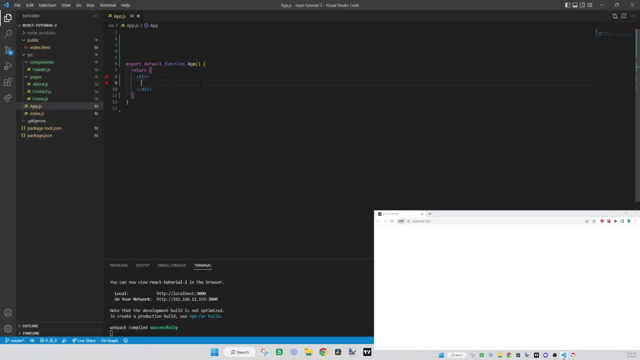 so what we're going to do is we're going to go over here to the app and we're going to import our router. so we already installed the router Dom, so we can just import it. so we're going to import browser router and then comma routes, oops, and then route from react router Dom. so now we've imported those. 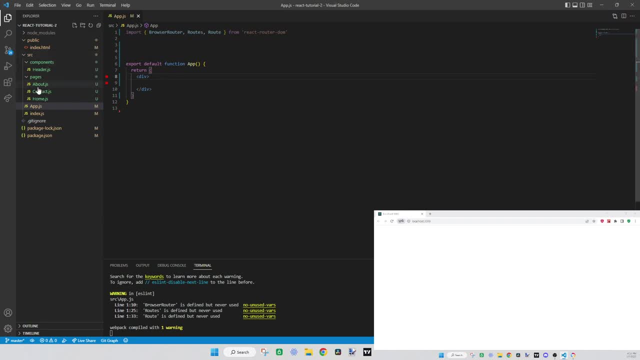 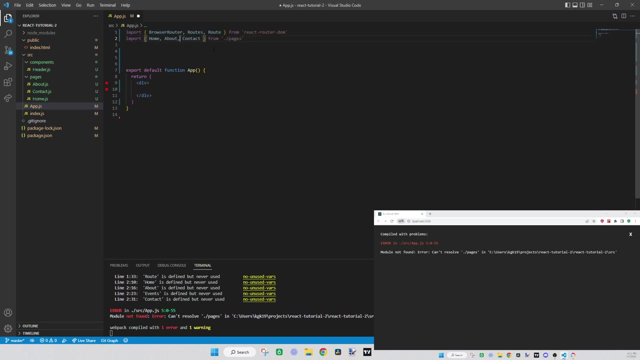 and we can use them in our code, but we also need to import these pages because we want to use those with the router, so in combination. I don't know what whoops 404 is doesn't actually exist, so does events, but there we go, it's actually. 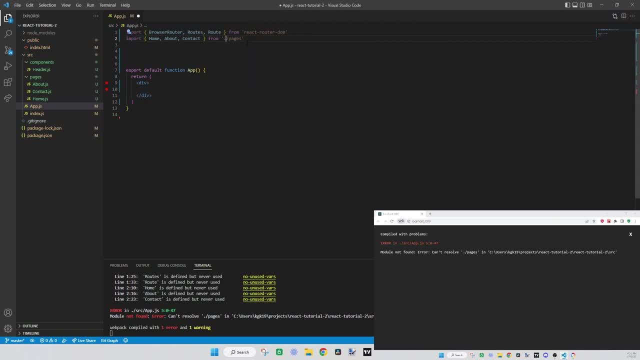 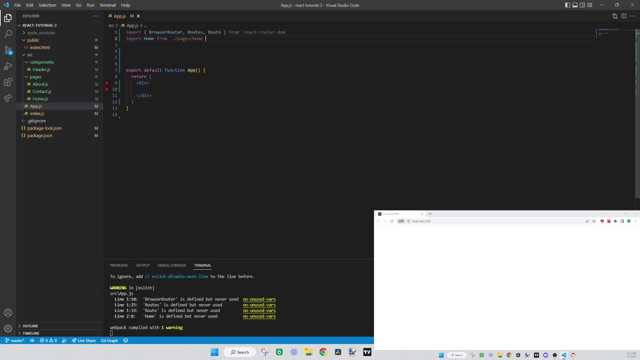 dot dot slash pages. actually, no, it's not. huh, I don't know. copilot thought that would work, I didn't think it would, so I guess I was smarter than copilot there. I knew you had to do this import about from dot slash pages about. so it's just like components pages are the exact same. 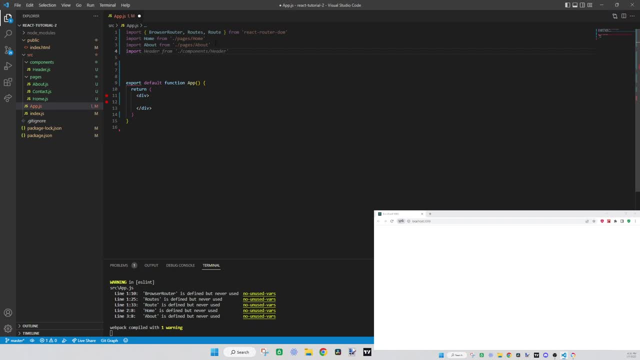 thing as components, as I'm sure you could probably tell, import contact from a slot path now. so we're going to go try that, the rice daughter, and now that's all we need to import. we can go start our routes. so to start off with we're. 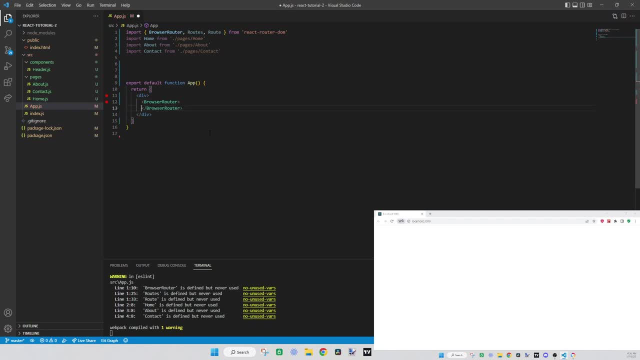 going to make a browser router and nest everything within this. see what it saying now: routes, and for some reason we have to nest everything within several routesиру eating back in a контрor, and for some reason we have to nest all of these in the browser because the 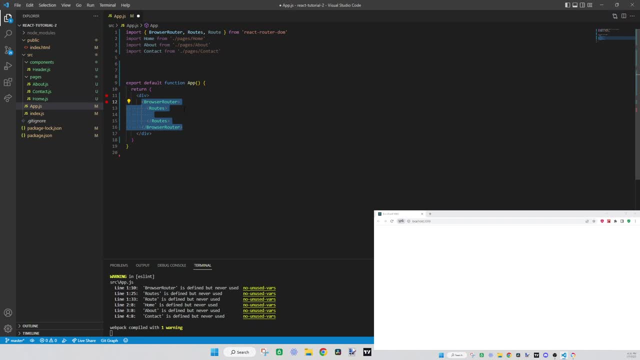 cation is not part of our system, so we have to use that to import all these routes so constantly. we have to place all the outputs, a lot of sites, in each of our nest it and both of these, both of these components. I'm not really sure why so. 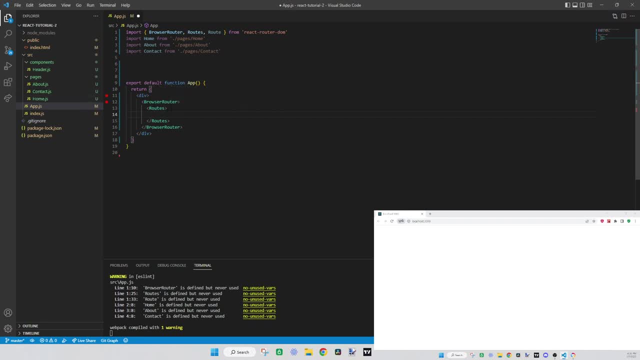 don't ask me, but that's how it works. if you just do routes or browser router, it's not gonna work. so now we're gonna create a route component and we're gonna make this one index. so by putting index here, what that means is: it's the default. 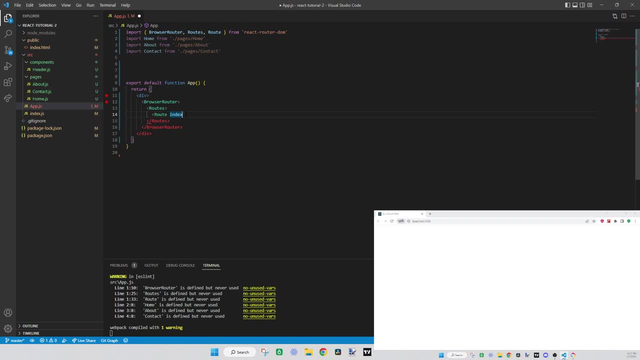 page that you're gonna load up to no matter. you know, if you don't have a URL path, you're just automatically going to be on that page. so this is usually what you want to use for your home page, and then we're gonna type. element is equal. 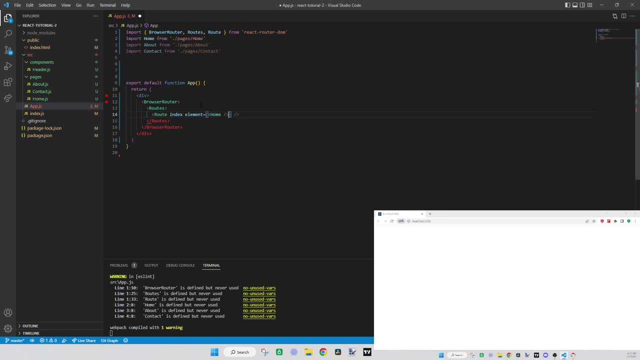 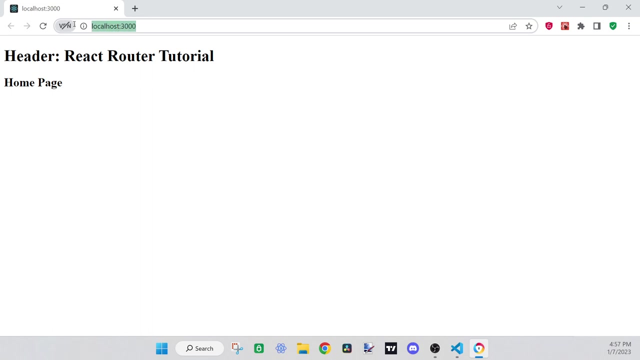 to home. you have to use the brackets there because you're putting a component. and then we got to close this tag. don't forget to do that. that'll give us an error. and so, as you can see over here, since we are, since we have no path, it is. basically the same as the previous one. so we're just going to close this tag and then we're going to close this tag. don't forget to do that. that'll give us an error. and so, as you can see over here, since we are, since we have no path, it is: 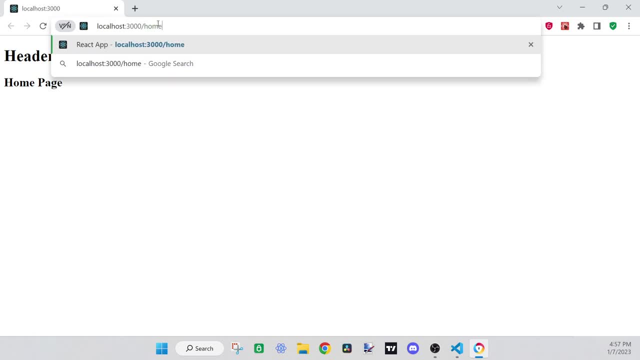 basically the same as the previous one, so we're just going to close this tag and showing us home. but now the problem is: if we type slash home up here, it's gonna show us nothing, because we don't have that path to find. all we have is index. 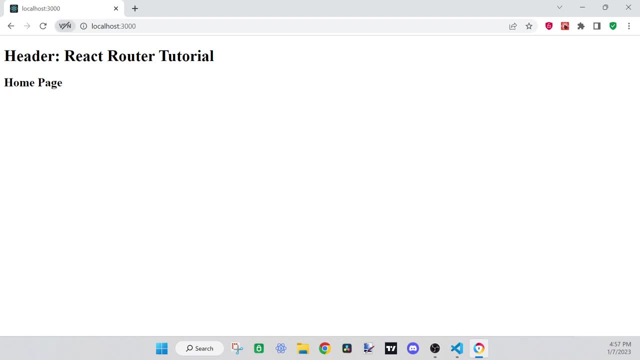 which means no path. so generally for home, you want to have slash home as a path to, just because it's just a little a little nicer to have that as an actual path as well. so now you can do path slash home, element home. so path is obviously what path you're going to, and index just means that there. 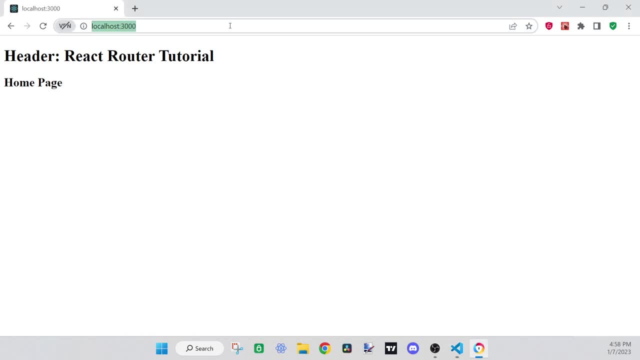 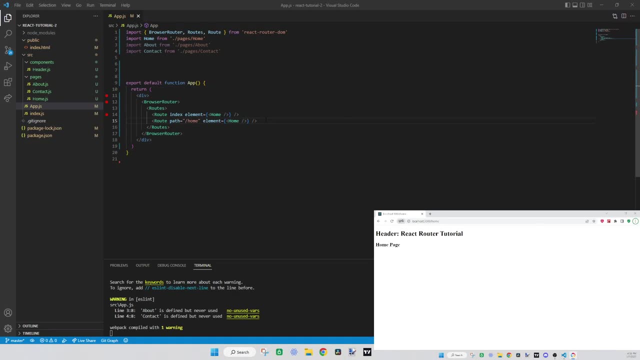 doesn't have to be a path like there is none. so now if we go over here and type slash home, it will be slash home. so sorry, I think I was on the other screen. I can't tell because I don't have a third monitor, but if you can see me type, 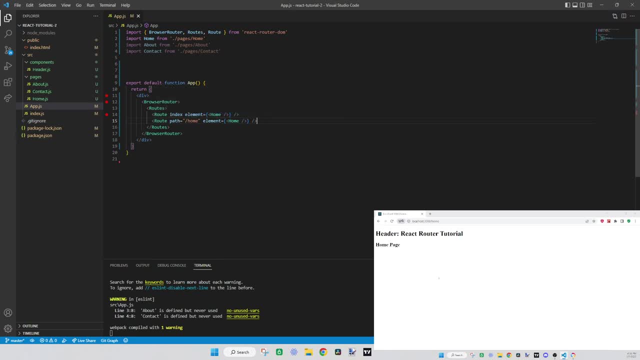 this, that's what I typed, yeah, anyway, so now let's make the rest of the routes with just the paths, so slash about, element about, and then route path contact. you have to make sure to do slash contact and then element contact, and you can also make like a 404 page. for that. you can make a new file, air 404. 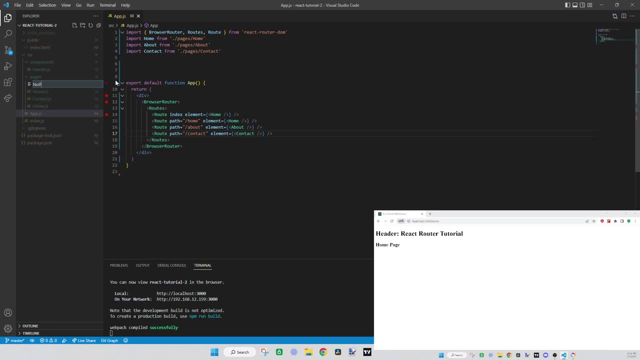 or you could- most people call it no page, dot j s, and then I'll just copy this: no, not this. there we go error, error 404, not found. all right, so now we can go over here and we can import no page from here and we can import no page from: 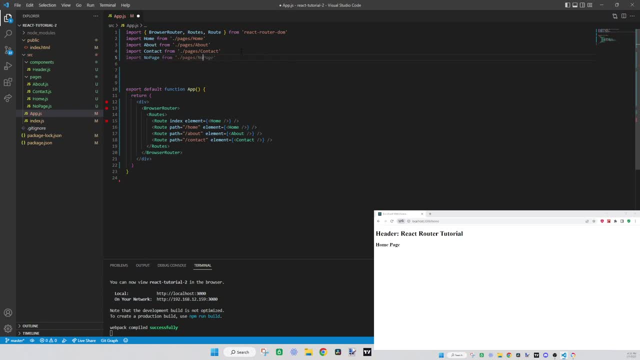 here and we can import no page from slash pages: slash no page. and now in slash pages, slash no page. and now in slash pages, slash no page. and now, in order to make this no page page show up. order to make this no page page show up. order to make this no page page show up. if the page doesn't exist, it's pretty. 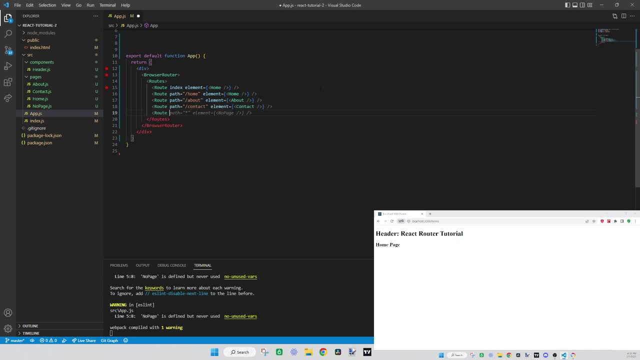 if the page doesn't exist, it's pretty. if the page doesn't exist, it's pretty simple. it's actually showing you right simple. it's actually showing you right simple. it's actually showing you right there: route path equals star element. no, there, route path equals star element no. 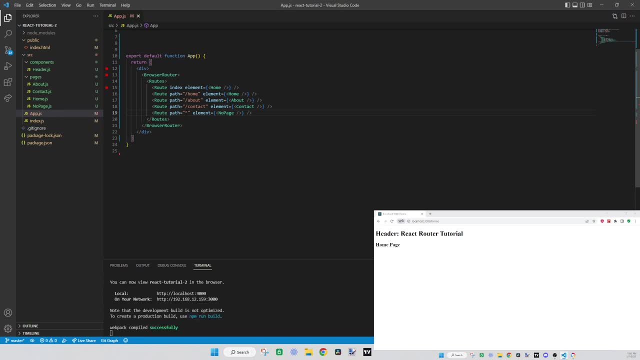 there, route, path equals star element, no page, and what the star means is anything page, and what the star means is anything else other than these. so really the star means all. just like in sequel, if you put a star, that means all of something. so by putting this no page last, it is effectively the last one to be seen. 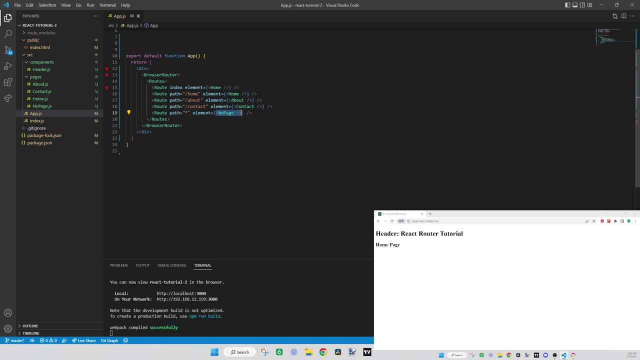 so it means if any path then go to no page, but all of these are going to be activated sooner, which means that you know if you have slash about, then you're actually going to be seeing the page. so you always want no page to be the last one, otherwise pretty sure if you have it up here. 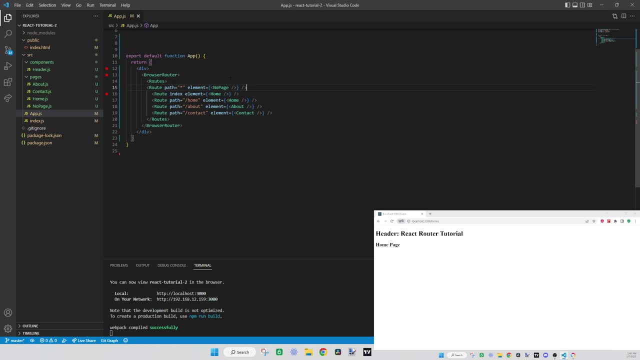 um, actually, i was wrong, i guess. i guess it works either way. um, you never know, with javascript i'm still learning myself. so here we are anyway. um, but that is how that works, though, with the all um, it's just anything other than what is already defined. um, so yeah. 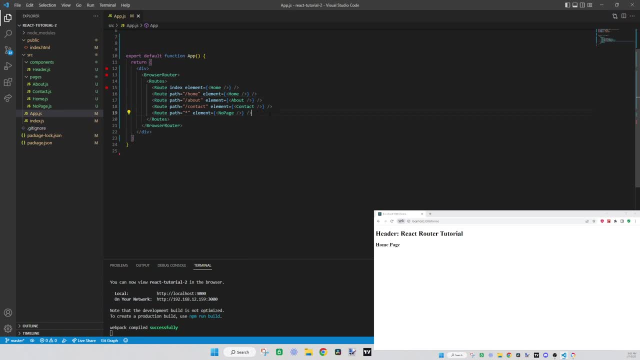 i think that's a specific component thing- is how that works with route. so i don't know a lot about the ins and outs of the actual router components. all i know is how they work. so anyway, that's pretty much all you need to know. i mean, you can go to slash home, you can go to. 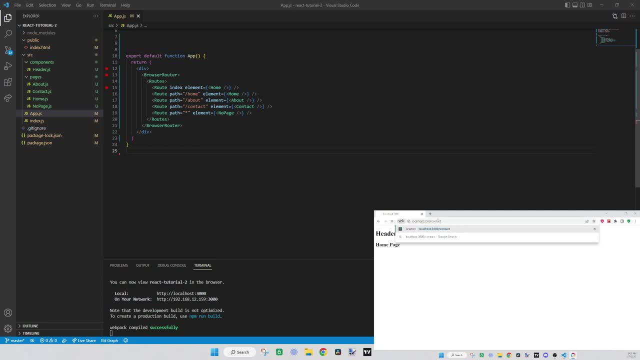 nothing that both shows you the home and then you can go to slash contact and that will bring up the contact page. you can have as much advanced uh styling and different components in there you can have. you know, you can make it look exactly like youtube and just have different pages for. 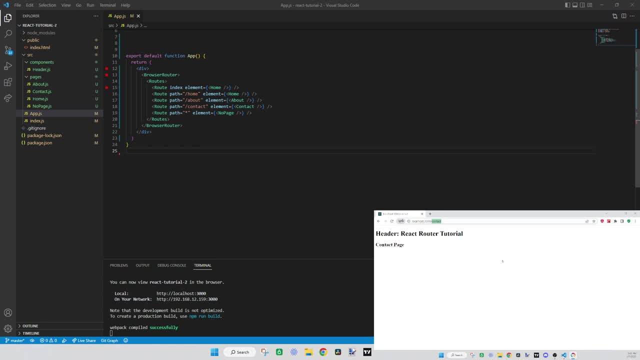 profile pages and whatever. you can make it very complex, and that's why react is very good for this, because, as you can see, i just made a bunch of different pages with routing and everything um very fast- honestly, i mean 10 minutes or so. um, you type about, it'll be about, so that's how. 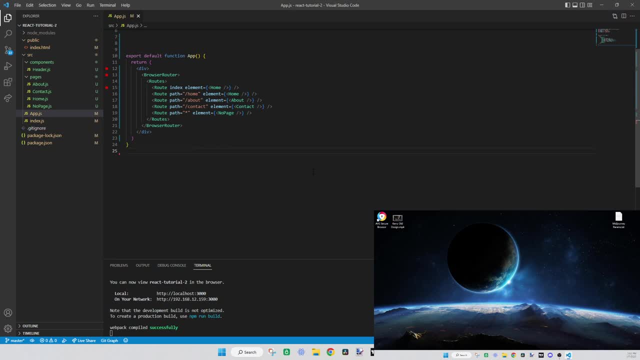 simple. it is, guys, really simple. this is why you need to know how to do it. you need to know how to people like react. it's not as hard as javascript, although it seems even harder. when you're used to javascript you're like: i don't know about react. you know it seems pretty complicated with.